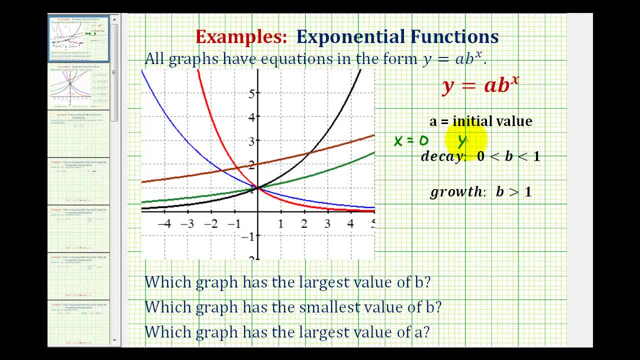 And determining y, a is also the y-intercept of the function. Next, if b is between zero and one or the base is between zero and one, we have exponential decay, which means the graph would be decreasing or moving down from left to right. so it would look something. 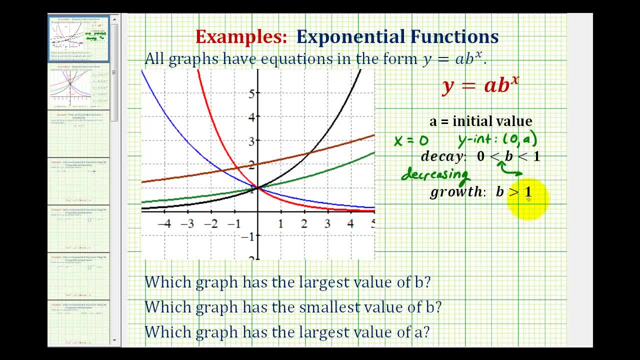 like this: And if b is greater than one, we have exponential growth, which means the graph would be increasing, which means, from left to right, the graph would be going uphill, looking something like this: Now let's go back and take a look at our questions. We 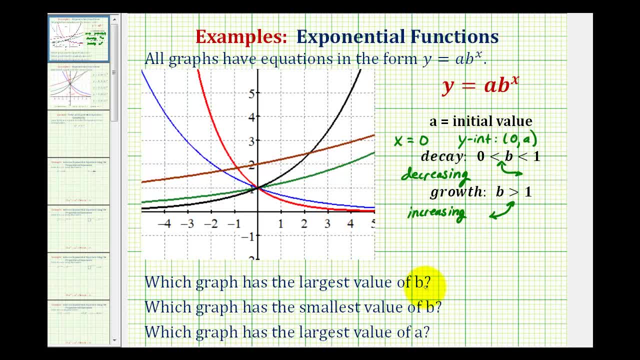 want to know which graph has the largest value of b. And again, remember, b determines whether we have exponential growth or decay. If we want the largest value of b, we only want to look at the graphs that are exponential growth or increasing functions, which would 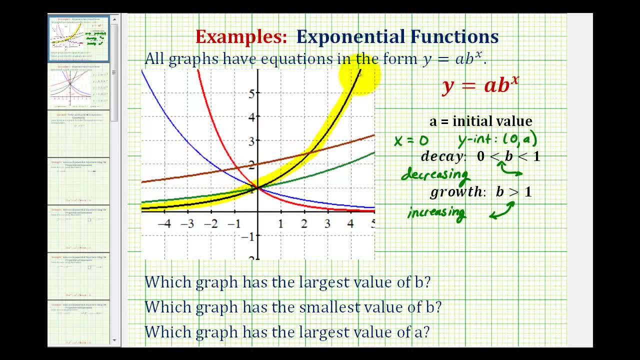 be this black function. here It's increasing, So b is greater than one, as well as the brown graph and the green graph. So the graph that's increasing the fastest would have the largest value of b, which in this case we can see. 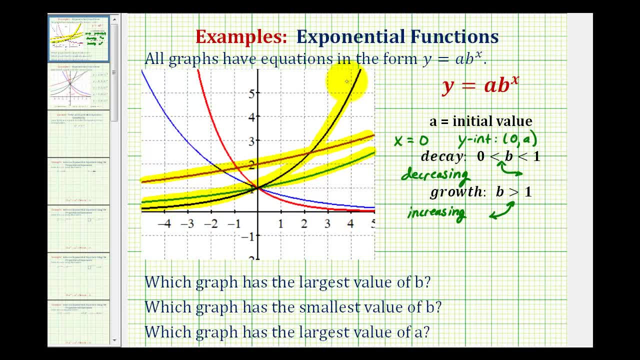 would be the black function, because it's going uphill the fastest. So this would be the black graph. Now we want to determine which graph has the smallest value of b, which would have to be a function that represents the largest value of b. Now we want to determine which. 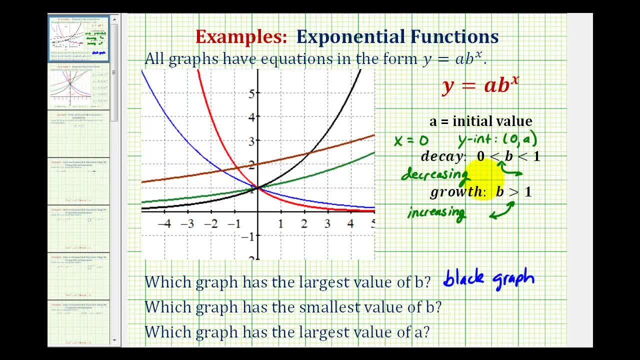 graph represents exponential decay or a function that's decreasing, which means now we want to focus on just the red graph and the blue graph, And the one that's decreasing the fastest is going to have the smallest value of b. Notice how the red graph is going downhill. 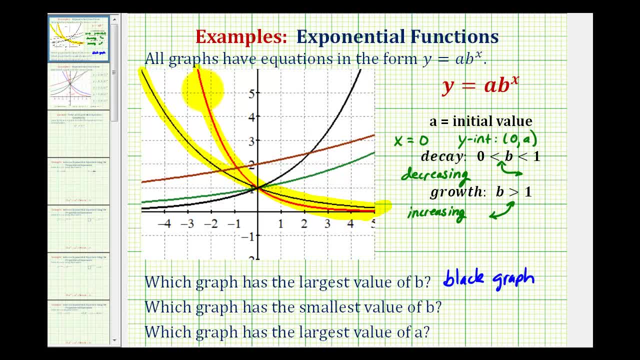 quicker or is steeper. Therefore it would have the smaller value of b. So the red graph has the smallest value of b. And then for the last question, which graph has the largest value of a? Remember, a represents the initial value, which would also be the y-intercept. So, looking at our graphs here,